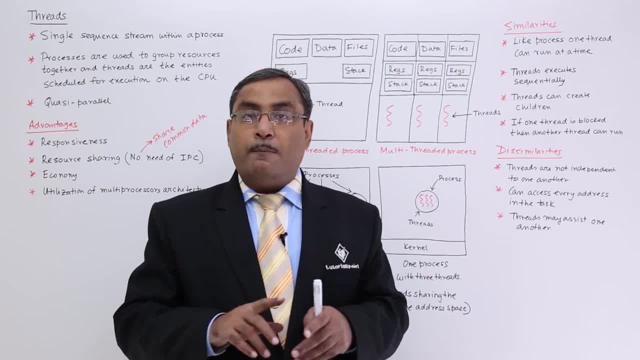 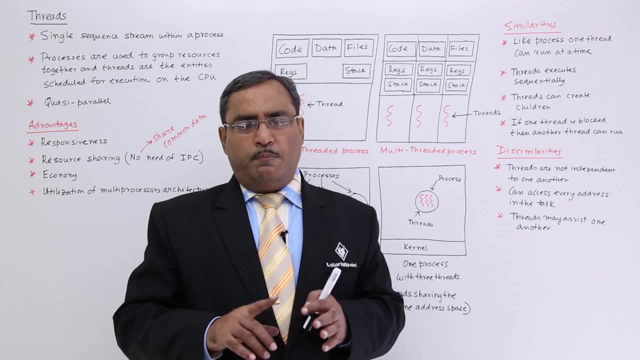 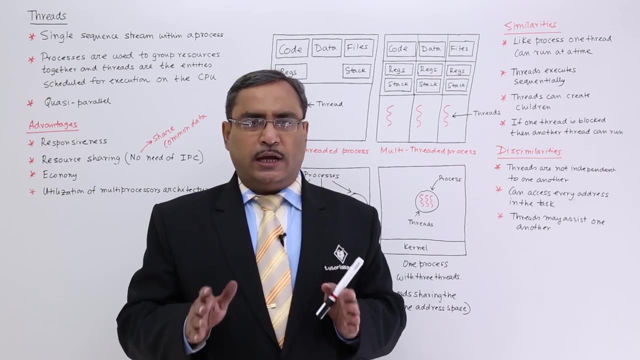 it seems that the threads are executing in parallel, but that is not true. they are executing in sequence. they are executing serially, but the context switching time will be done in sequence between one thread to another. thread is so small and the context switching is taking place in a such a fast way so that it seems to be a quasi parallel. ok, now what? 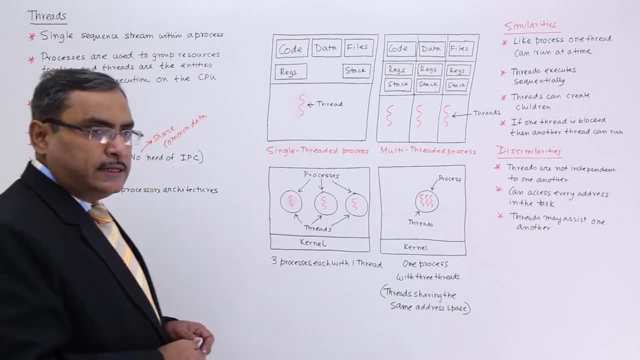 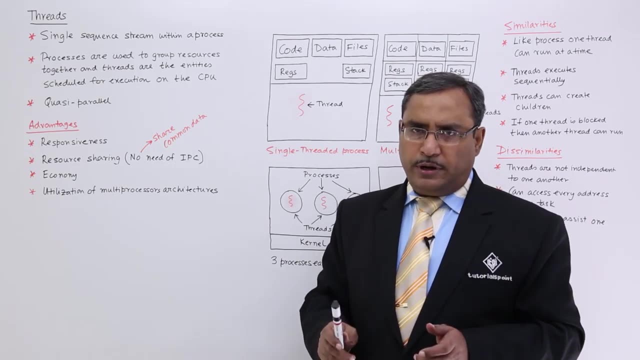 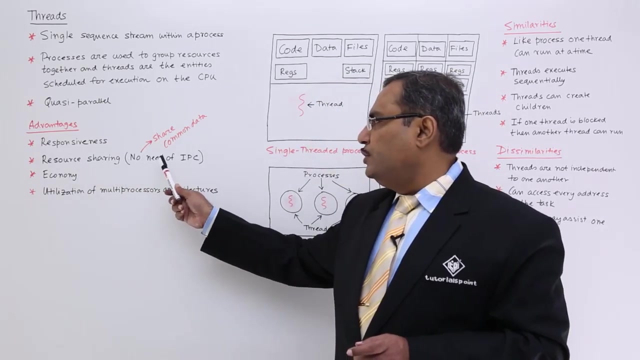 are the advantages of using a thread: the responsiveness. just now i have defined this particular terminology. that is a responsiveness. that means the context switching time between thread is very small, very low, as if they are executing in parallel resource sharing. no need for any inter process communication. there is no need because they are not the separate. 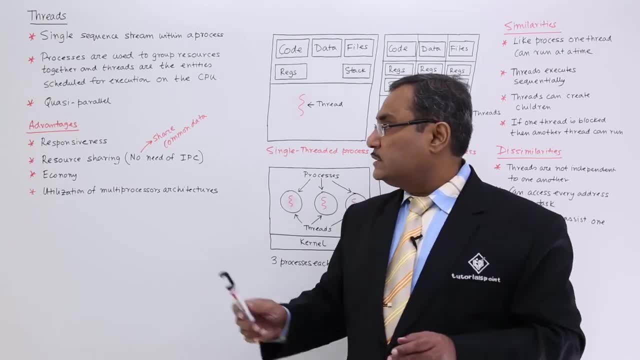 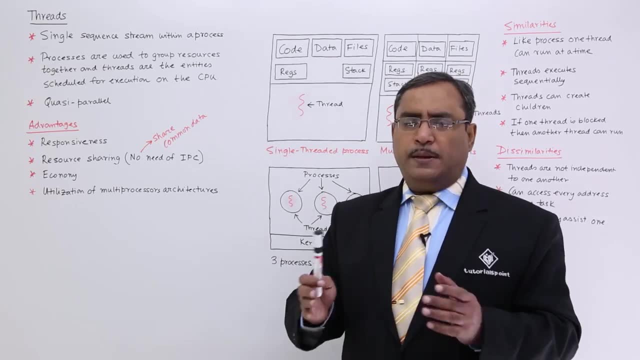 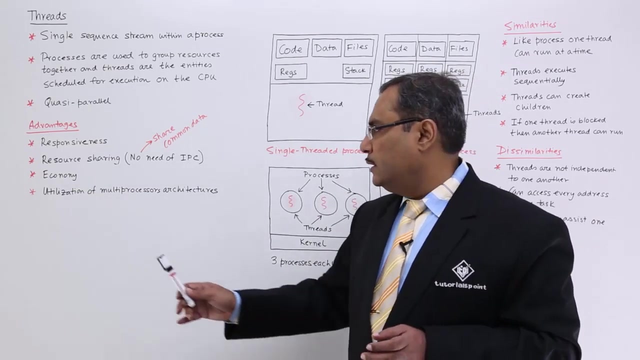 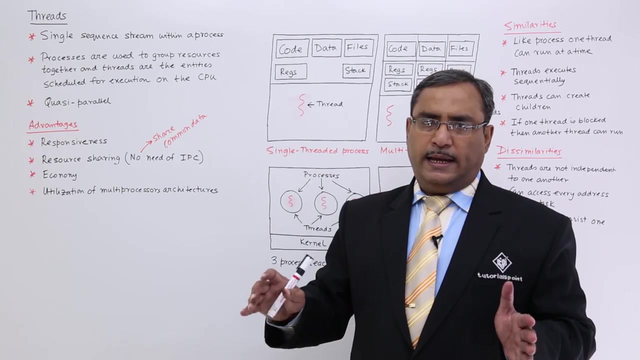 processes. all of them are existing within a same process and share the common data economy. we are not going to allocate a separate memory space, separate program code or say separate global data. it does not require so thread execution will be economical. utilization of multi processors architecture. so whenever we are having multiple processors in a certain 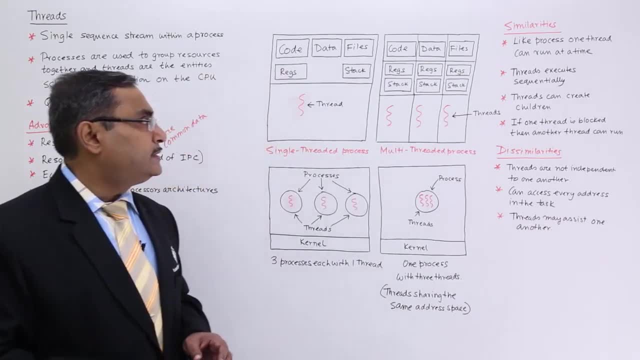 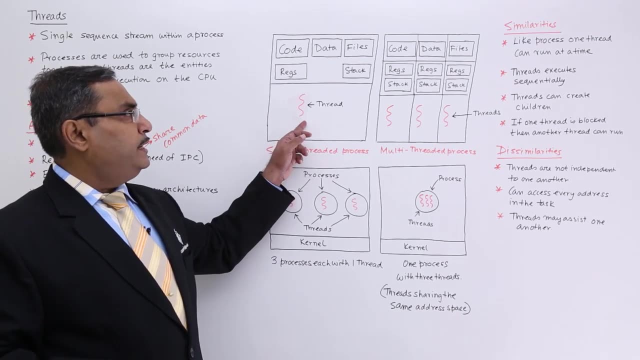 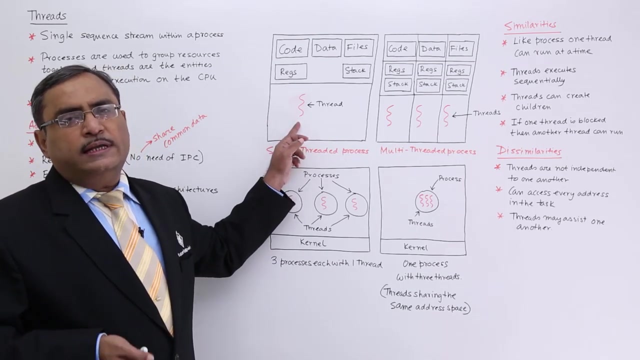 system, then thread execution will be easier. in that case, single threaded process, that means here this process is having a single thread, so this particular thread is having this registers and stacks which are dedicated for this particular thread, but as here we are having only a single thread, so no question of any kind of dedicated or sharing the terminologies. 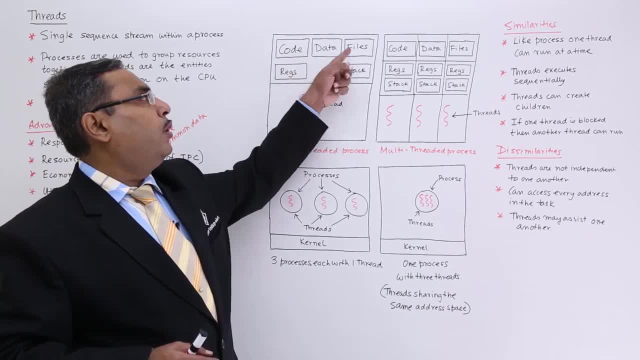 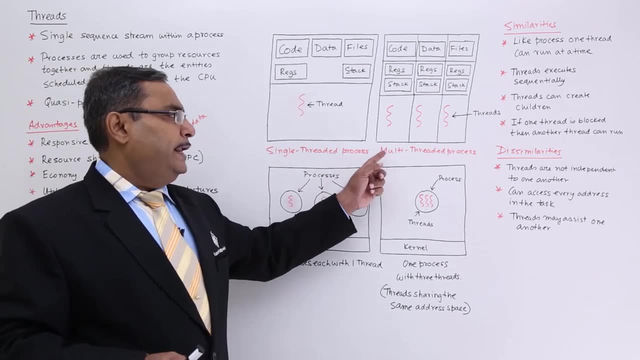 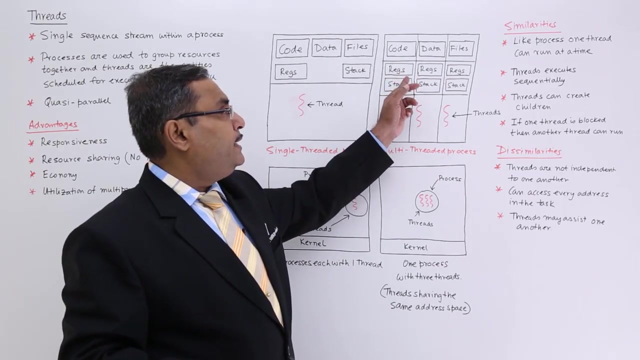 are not very much useful here, because this thread will be using all these resources and residing in this particular system Memory area. so single threaded process. in case of multi threaded process, for each and every thread, as I discussed earlier, they will have a separate dedicated. they will have a 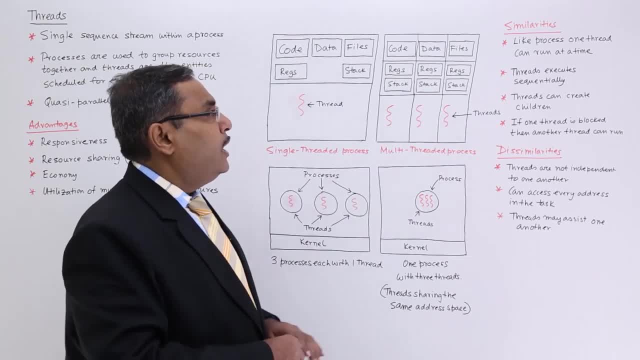 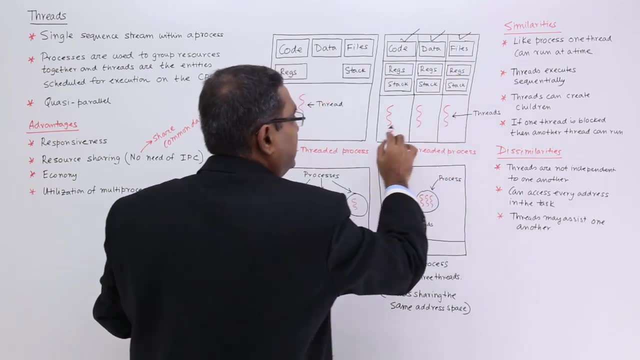 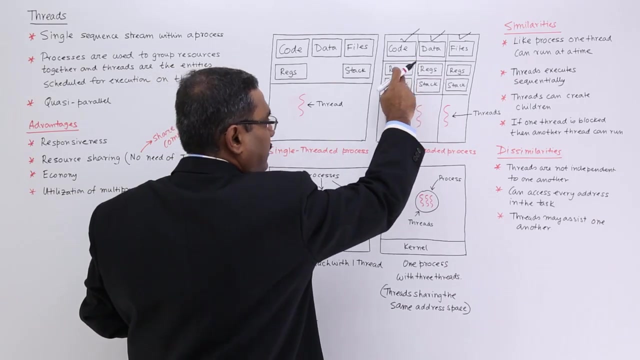 separate dedicated registers, stacks and so on, and this particular code data files. this particular code data and files will be accessed by all the threads at the same time, will be accessed by the all the threads at the same time, but this registers and stack will be dedicated for them. so that is why I am having three threads. so I have written this registers. 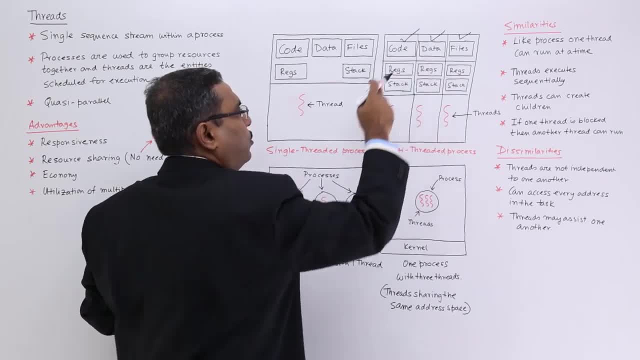 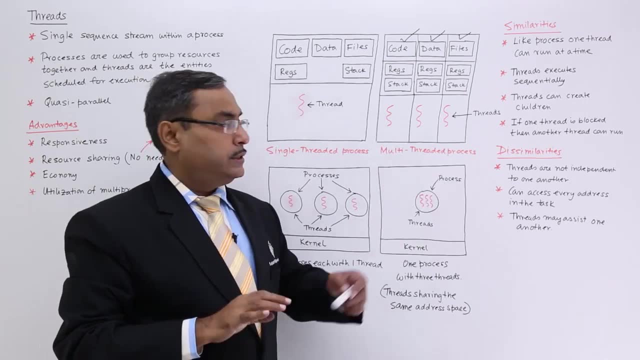 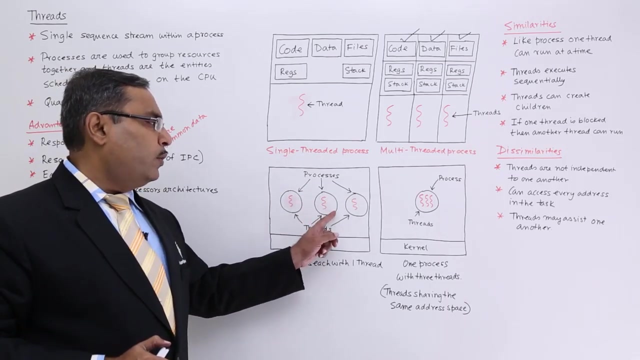 and stack three times for each one of them. but this code, data and files- I have written them once because they will get shared. so that is known as multi threaded process. Now a process we are having three processes are there. each process is executing one thread at a time like this. so we are having three processes. each process is having a single. 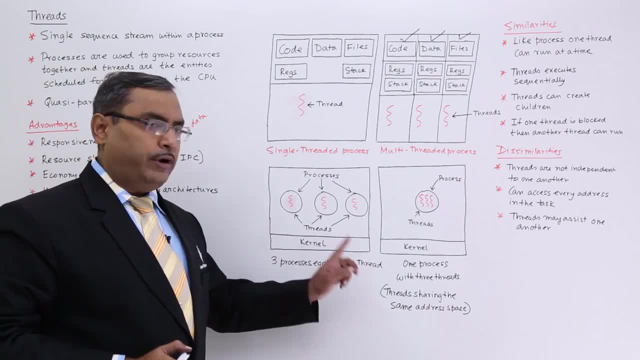 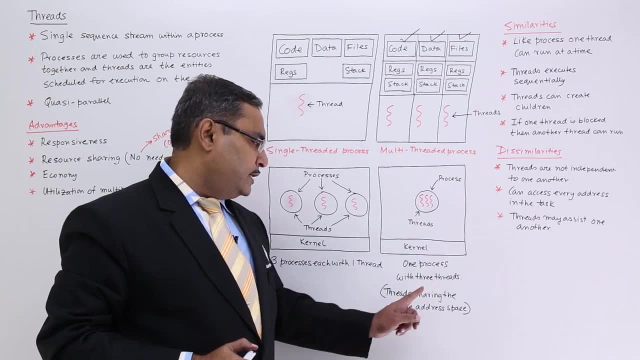 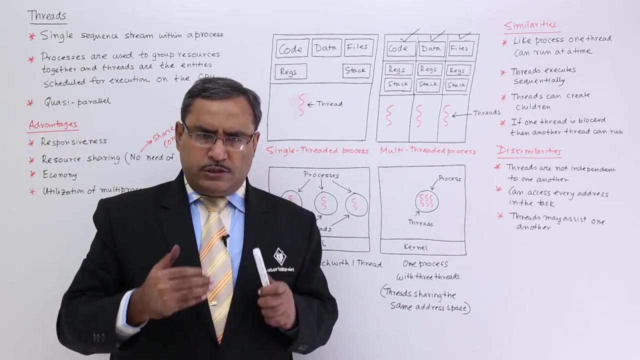 thread. So three processes each with one thread. but here you see there is a single process and it is executing three threads. so with three threads and thread sharing the same address space as I have mentioned. Now question is coming in mind particularly: what are the similarities and dissimilarities? 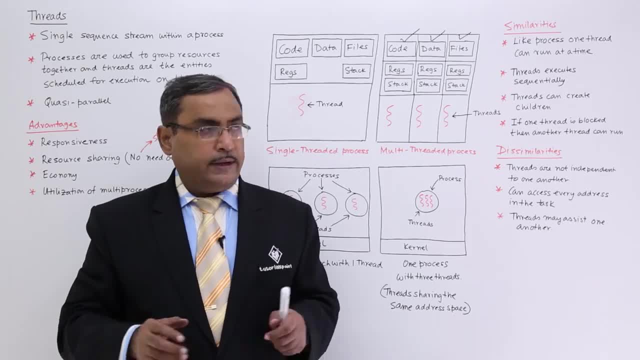 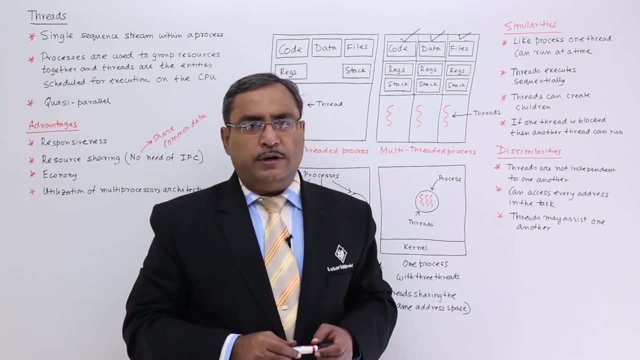 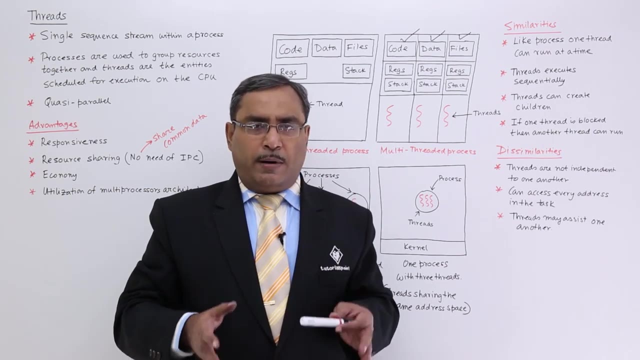 between a process and a thread. it is a very common question. the similarities are like, like process, one thread can run at a time. I told you that threads will be seems to be parallel execution because the context switching time is very low, so it is quasi parallel. but actually, like processes, it will. 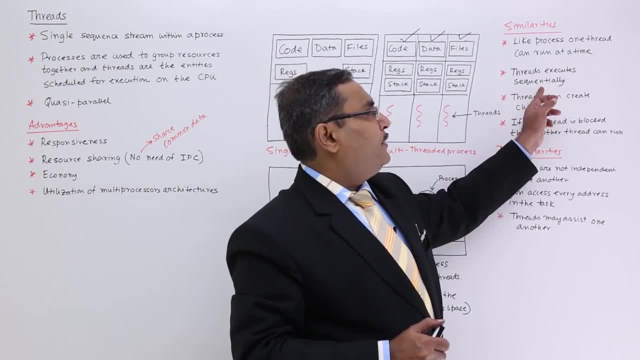 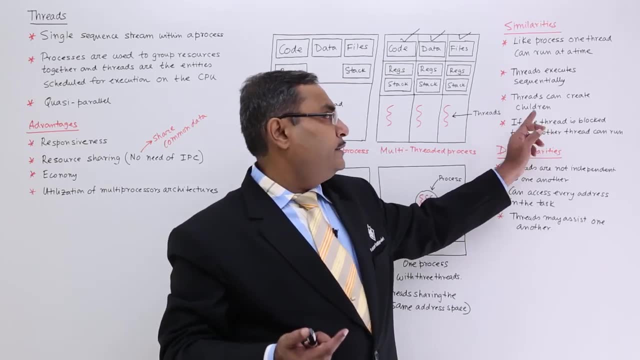 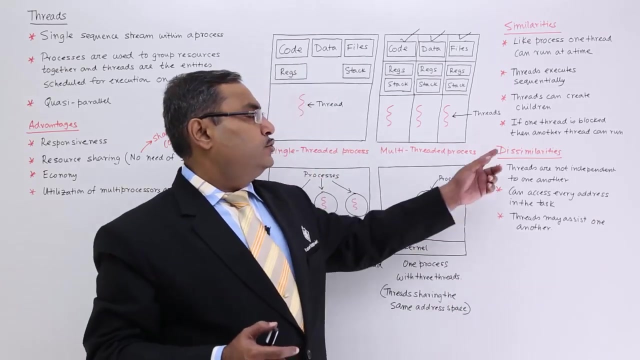 be executing in. serial Threads execute sequentially like a process, so there is a similarities threads can create a children- child thread can be created. if one thread is blocked, then another thread can run, so they can work independently. So that is also common in case of processes. process dissimilarities. threads are not independent to each other. they are dependent on each other. so they are not independent because they have got created and residing within the same process. memory area can access every address in the task. so one thread memory space can be accessed by the another thread memory space. so the memory spaces are not protected. but in case, 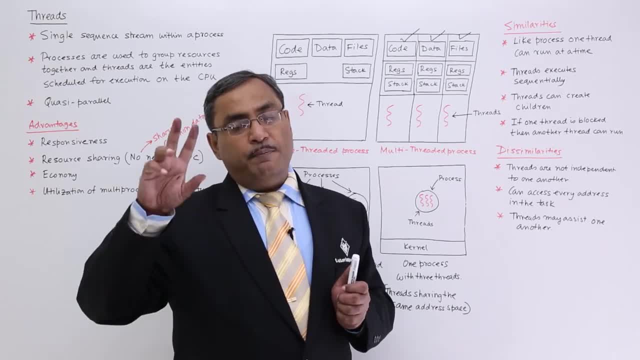 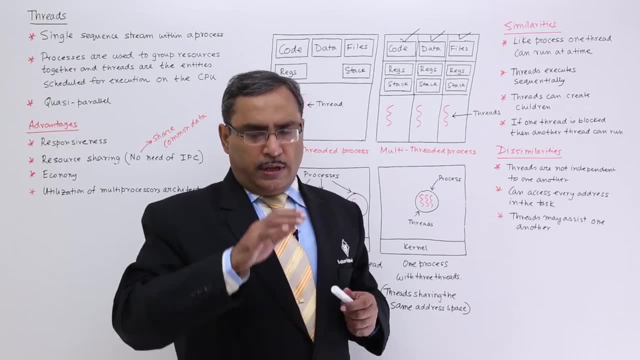 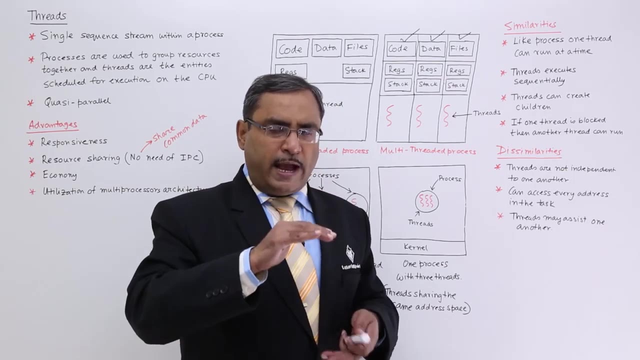 of process one process, one process cannot access the memory space allocated by the another process. if it wants to do that one, then that is known as a protection error, because each and every process has got its own memory space allocation and that memory block should remain protected from being accessed by the other processes. threads may assist one another in. 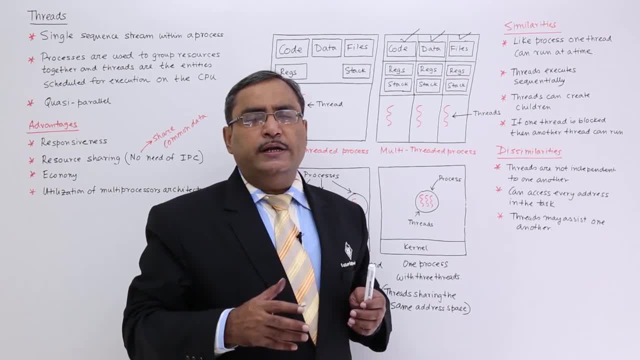 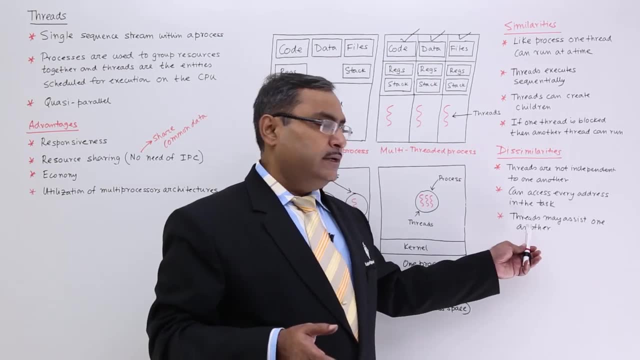 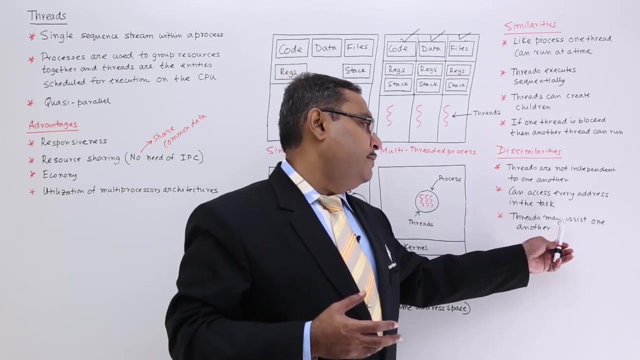 case of process, you see, different processes are being created by the different users, so one process is helping another process may not be true, but in case of threads, as all these threads within a single process they are, they are getting created by the same process, so one thread may assist the another one. so these are the dissimilarities between a process.